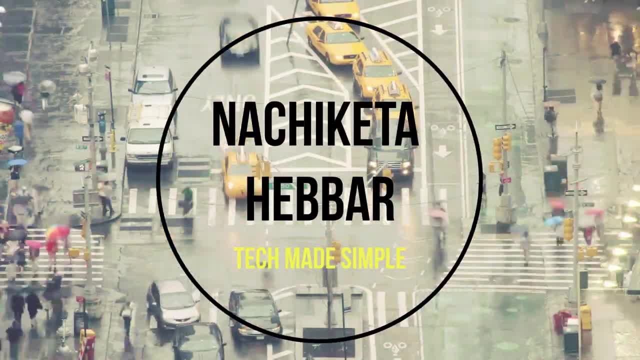 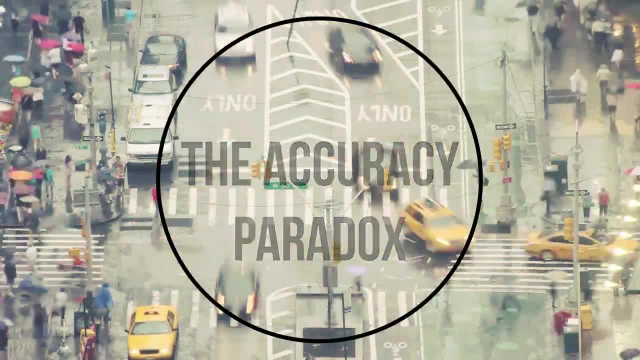 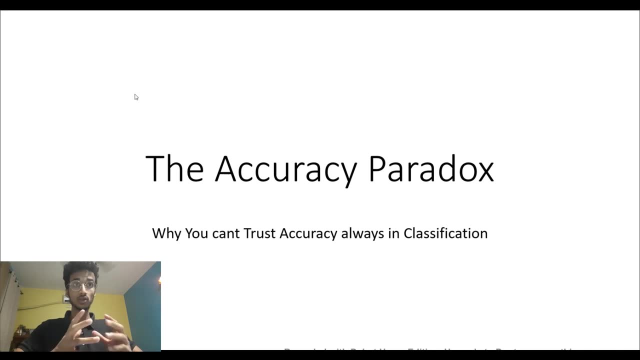 So, hi guys, welcome to my channel. My name is Nachiketa and in this video I'm going to talk about the accuracy paradox, Basically why in classification problems, you cannot trust the accuracy always. Even if a model has 99% accuracy, that does not mean it's good, And I'm going to 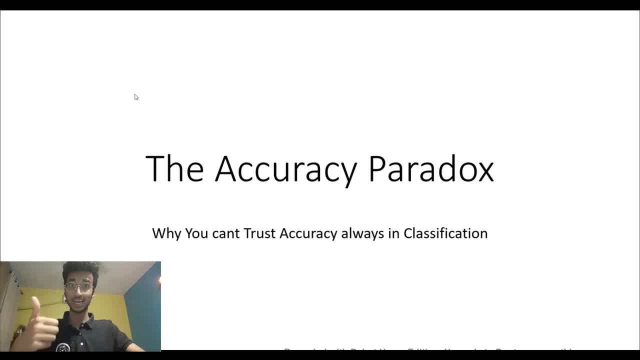 show you how right. First of all, let's start by defining what accuracy actually is In statistics. basically, accuracy is the correctly classified case divided by total cases. right? This is definition. So let me show you an example where this definition is going to give you a very bad 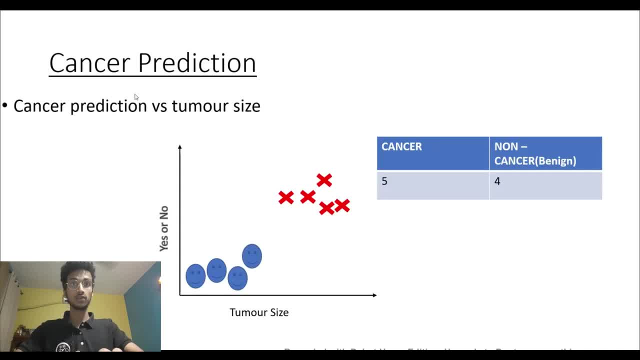 result. So look at this case right. Basically, we're predicting if a particular tumor is cancerous or not based on the tumor size. right? You have the tumor size on the x-axis and you have the results on the y-axis. These blue smileys are basically: 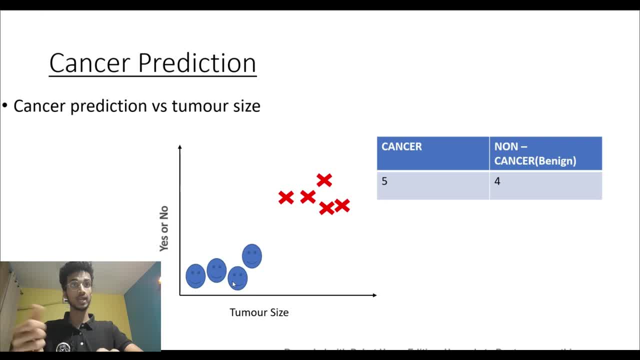 non-cancerous tumor cells, which are also called as benign, and the red cross is cancerous. So this is a pretty good data set, right? We have four examples for non-cancer and five examples for cancerous. However, consider this data set. So in this database you have four smileys. 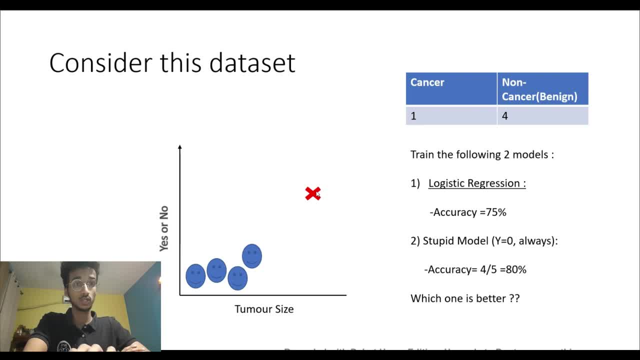 which means you have four non-cancerous examples and one cancerous tissue, one cancerous tumor, right? So this is a very bad data set. It's not even related, It's only distributed. So say, you train the logistic regression model and you've got an. 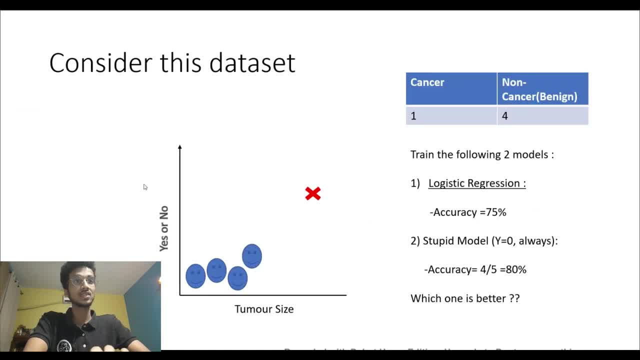 accuracy of 75%. right And say this is a very stupid model which is blindly predicting any given tumor as non-cancerous without even looking at it. However, in this case, that would give you an accuracy of four out of five because, anyways, in the five examples in the data set, four are 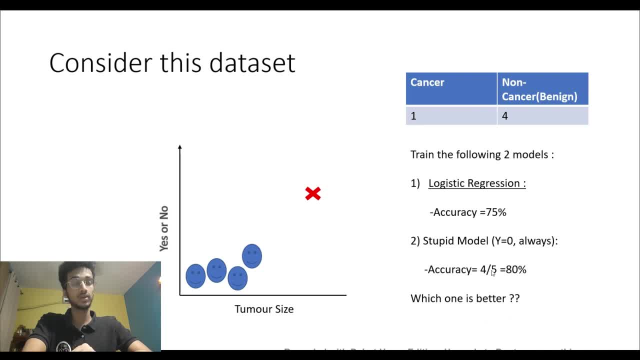 anyhow non-cancerous. So if you blindly predict non-cancerous, you're going to be right four out of five. Similarly, if you had a hundred examples out of that, 99, say, were by default non-cancerous, then even a stupid model would be able to get an accuracy of 99%. That is a big problem. 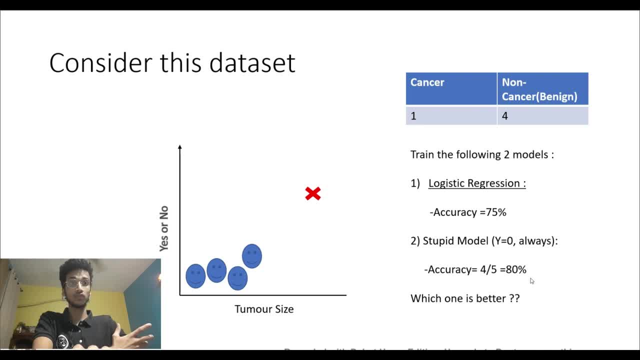 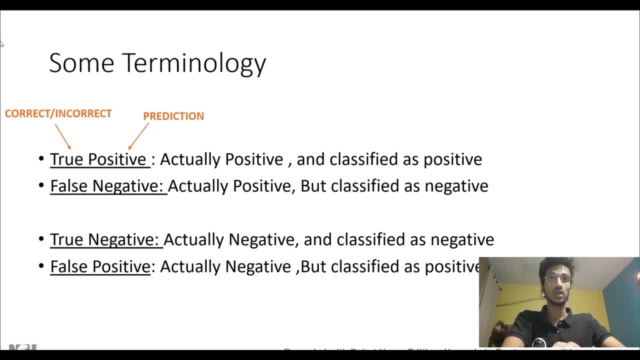 We cannot trust the accuracy because it's largely dependent upon what kind of data set you were using, So that for that we introduce some new terminology to counter this problem. First, is true positive, which is basically an prediction, which, uh, basically, uh, uh. 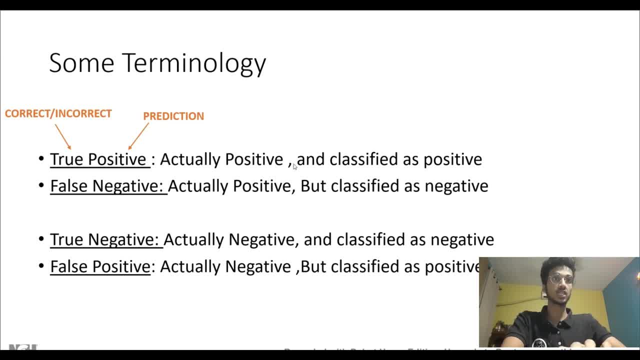 basically a sample which was actually positive and also classified as positive. False negative is one which was actually positive but it's wrongly classified as negative. Similarly, true negative is one which is actually negative and also classified as negative. and false positive is one which was actually negative but has been classified wrongly as positive. 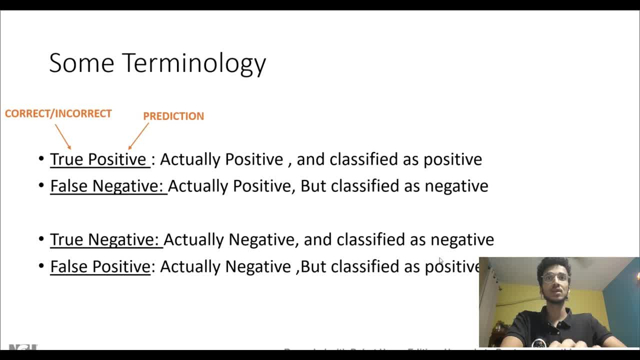 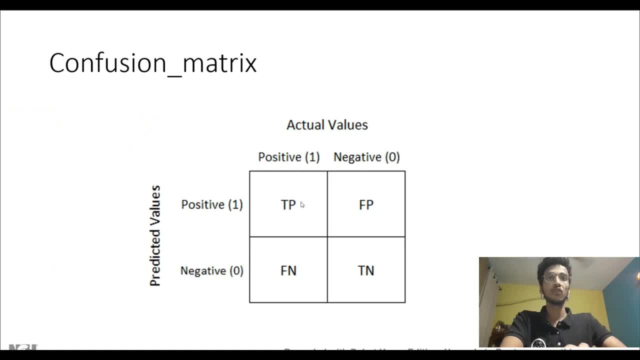 right, And using these four terminologies, we build something which is called as the confusion matrix. You might have seen it in the previous video, You might have seen it in a lot of places, which is nothing, It's just a presentative. 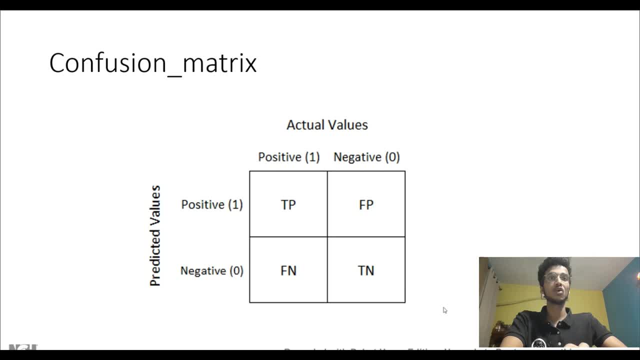 of your true positives and true negatives in a diagonal manner, and false positive and false negative on the opposite diagonal. So you can probably say that, uh, two positive and two negative should always be maximum, because those are the predictions which are actually correct, right? So now that we're abandoning accuracy, we've decided that accuracy 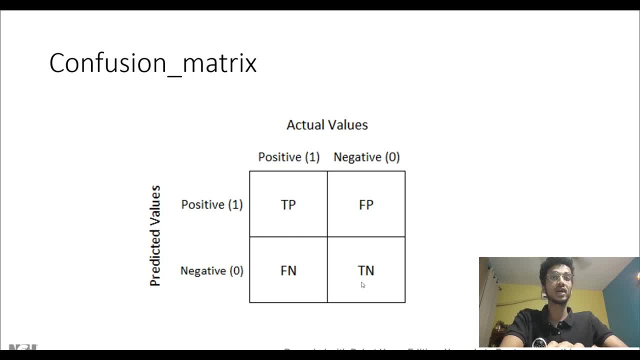 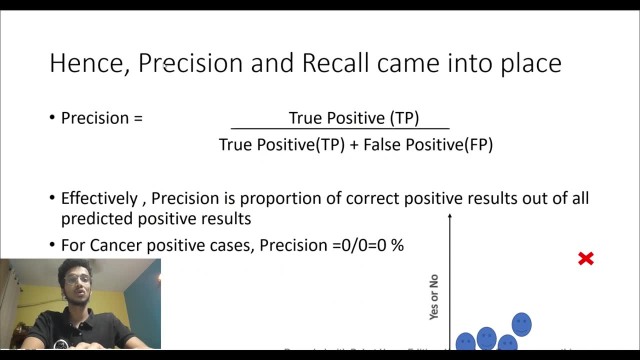 is not good. So what do we depend upon? right, For that, we have created some new definitions, which were brought up specifically in the previous video, Specifically for this issue, which is called precision and recall. Let's look at precision: Precision is nothing but your true positive divided by true positive plus false positive. 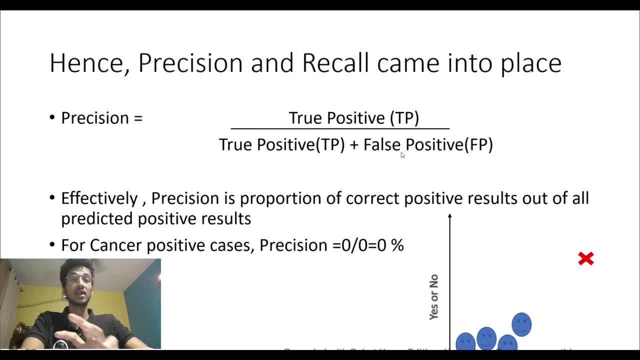 People get confused by the definition, by the formula. Just understand the meaning, right? Precision is basically a proportion of the correct positive results out of all the predicted positive results, right? So for all the cases in which your machine learning model is saying that it is a cancerous, 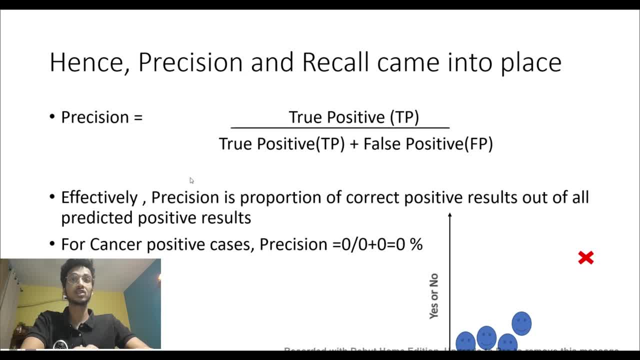 How many of them were actually correct. So for in this case, for cancer positive cases, precision is equal to in the numerator we have zero because not even a single cancer case was classified correctly, because a stupid machine learning model was saying that every tissue is non cancerous. So true positives are zero divided by the true positives plus. 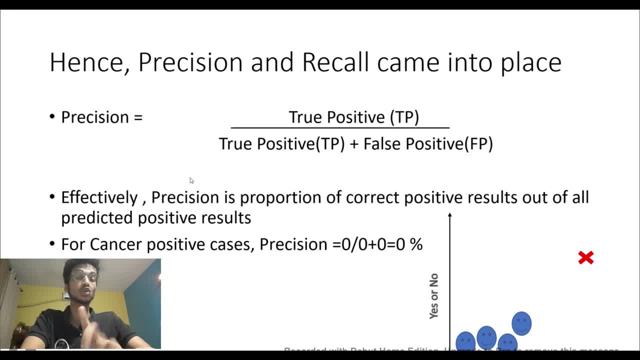 false positive, right, False positive here is also zero. Why is it zero? False positive is nothing. It is those which are actually negative, but classified as classified as positive. In this case, our machine learning model is stupid. Blindly it is calling everyone as negative. 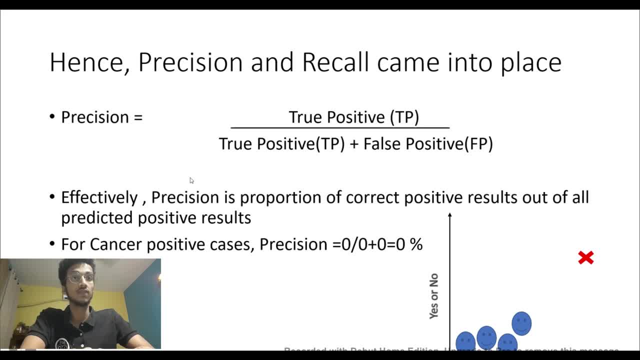 It is saying that all the cells are non cancerous. So we have zero by zero, which is 0%, right. So, on one hand, when we were getting an accuracy of 80% for the same case, our precision has become 0%, right. So that is, uh, this is a good indication, right, That our machine 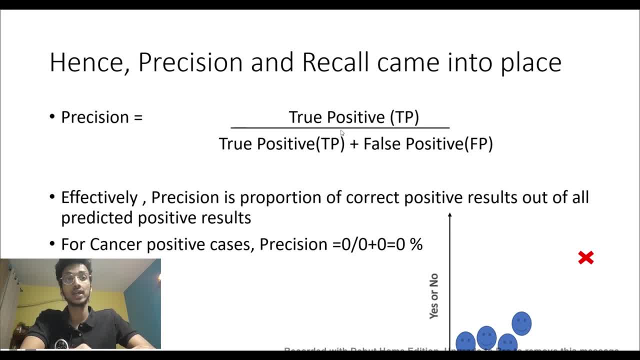 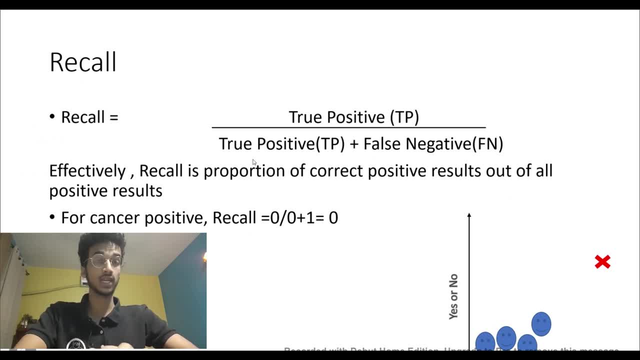 learning model is not as good as false positive. So one might have thought by simply looking at the accuracy formula that we use in. this is called a recall, which is simply but the true positive divided by true positive plus false negative. right, This is almost same as precision formula, but instead of false. 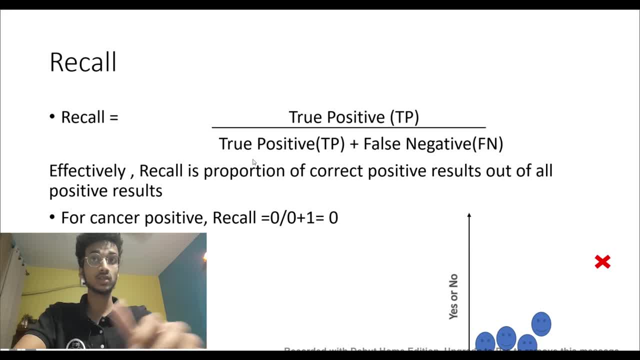 positive in the denominator we have false negative. What that does is makes recall the proportion of correct positive results out of all the actual positive results. Precision was a little different. It was the correct positive results out of all the predicted positive. So for the cancer positive cases recall is equal to: we have zero in the numerator as 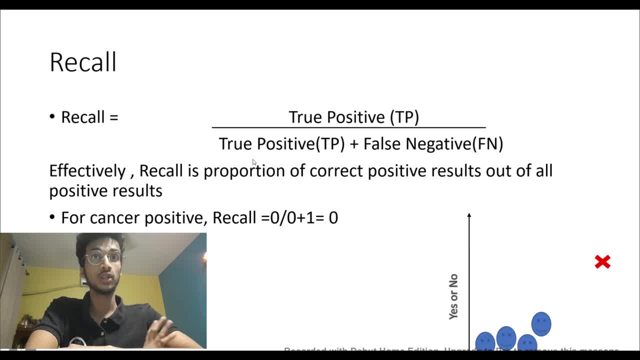 none of the cancer cell were identified correctly. The denominator we have true positive as zero plus false negative, which is one. false negative is basically: uh, something which our machine learning model is saying as non cancerous but was actually cancerous. So we have basically: 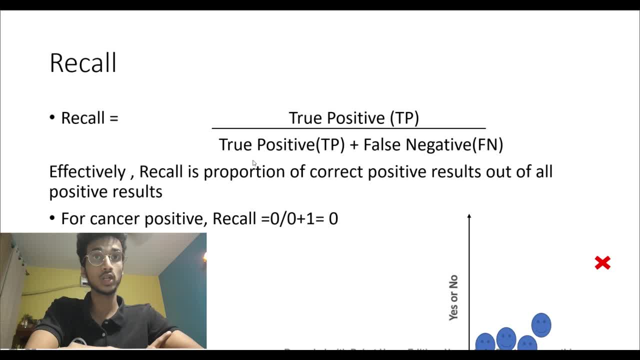 one misclassification, which is, uh, written in the denominator. So we have zero upon zero plus one Right. So we have precision zero, recall zero, which is a indication that the machine learning model is indeed stupid and we should not rely on the accuracy. So, uh, combining the precision, 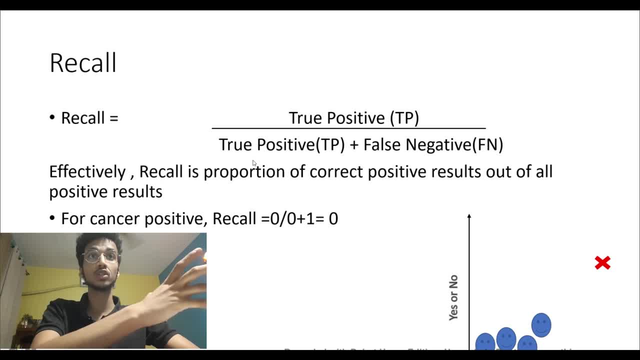 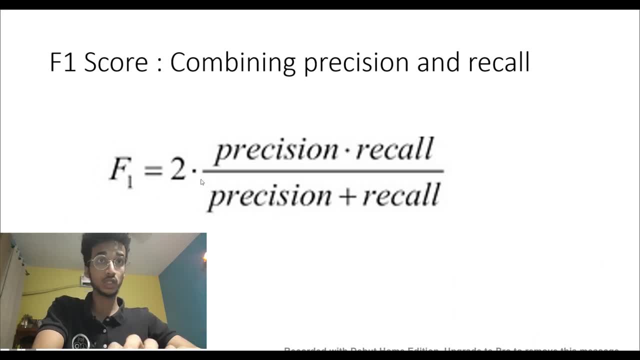 and recall, we come up with the final measure, which is called as your F1 score, Basically just a harmonic mean of your precision and recall, defined as two into precision, into recall, divided by precision plus recall. So in classification we do not simply trust the 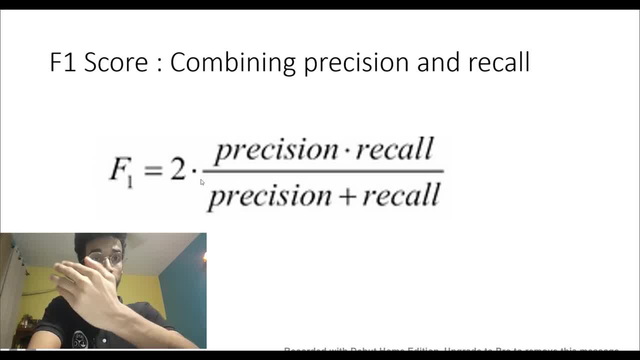 accuracy. We also check the F1 score right For all the classifications that it's making Right. For example, if a machine learning model is classifying digits into 0,, 1,, 2,, 3,, 4, up to nine for each label, for 0,, 1,, 2,, it will separately calculate the precision recall. 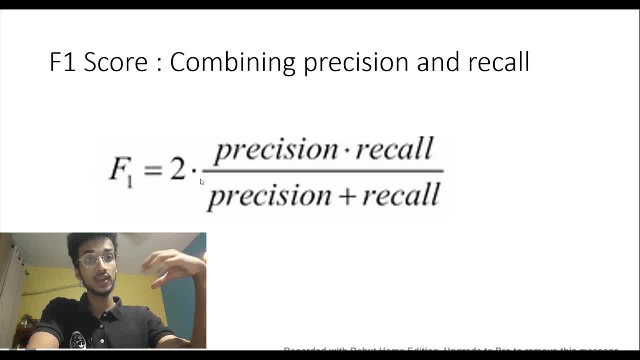 and the F1 score And you will check that and find an average F1 score for all labels And using that you will be able to decide whether your model is indeed good or not. So the benefit basically is that your F1 score is not dependent on how bad of a distribution.